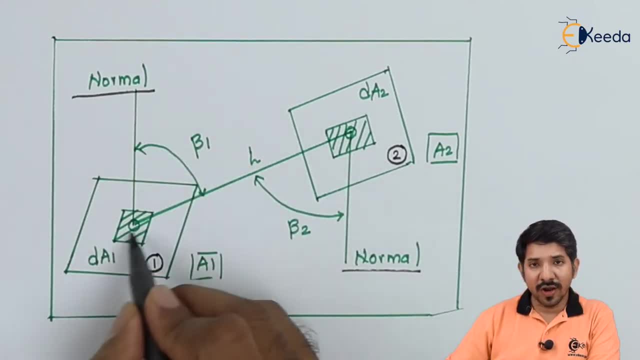 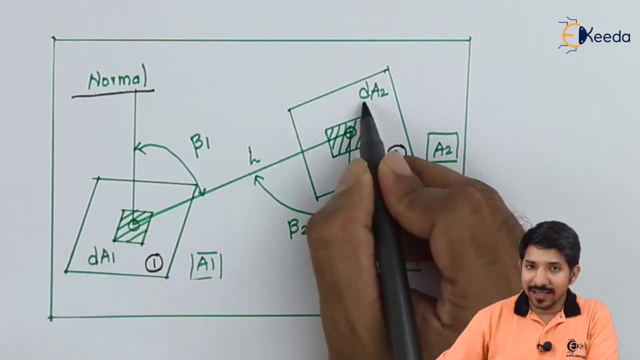 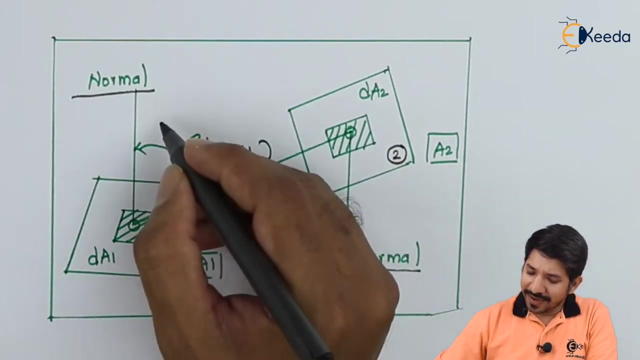 the normal drawn to the small elemental area for the two different surfaces. Now these small areas are nothing but DA1 and DA2.. Now let us draw some angle or a line. Let us say the length of the line is L joining the two small elemental areas DA1 and DA2.. Now this will make some angle with the normal. 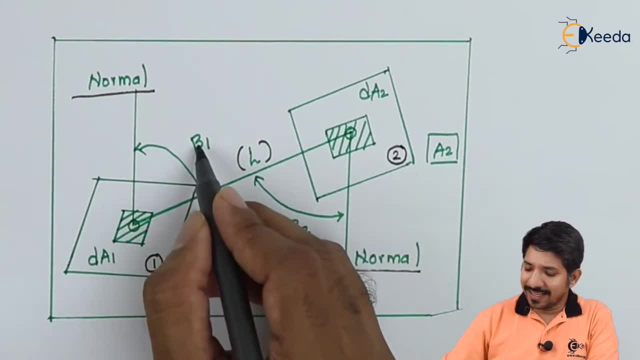 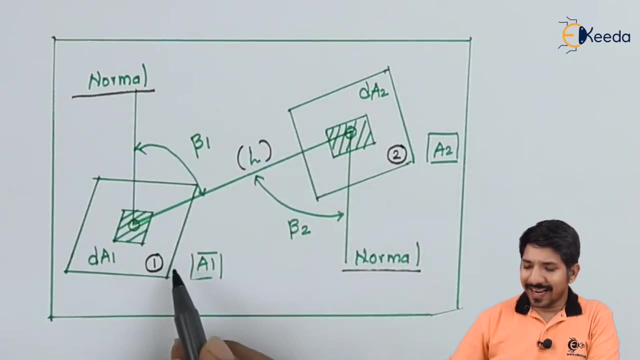 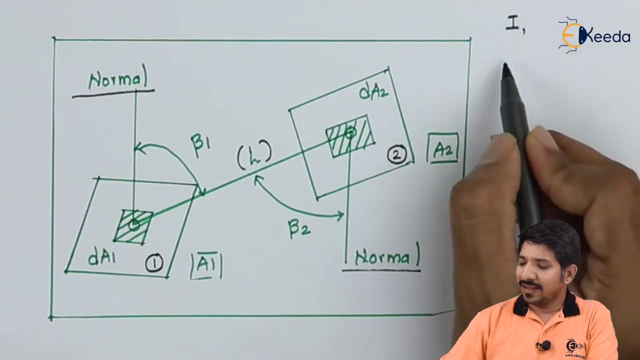 for surface 1 and surface 2.. Let us say the angle is beta1 and beta2.. Now, with this geometrical construction, let us try and find out the amount of heat that is transferred from one body to another body Now, for which we will be required the knowledge of intensity of radiation, that is I. Then 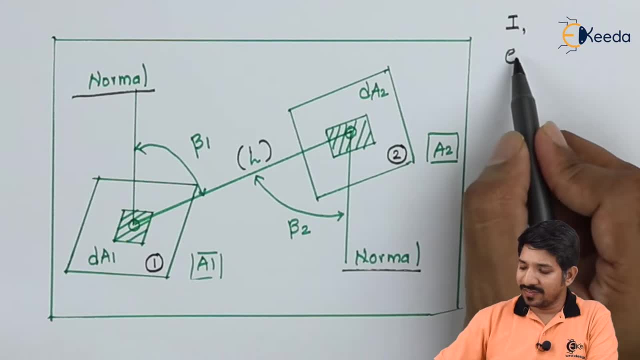 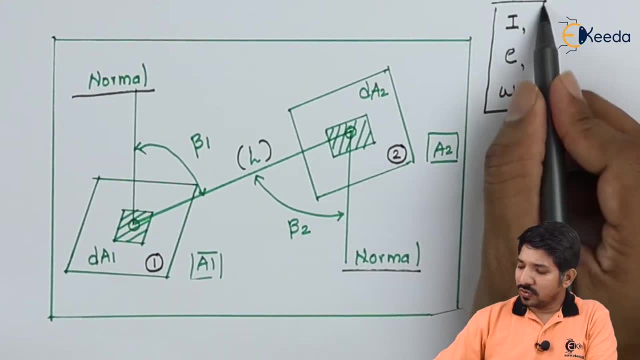 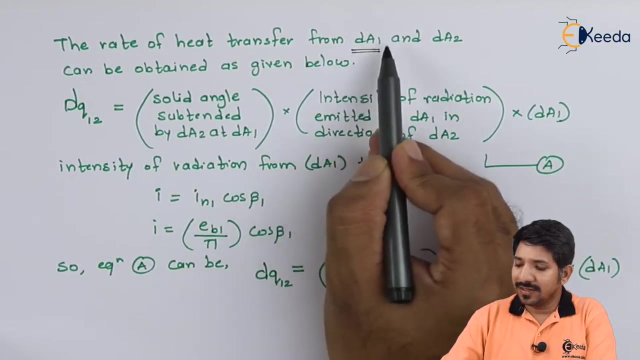 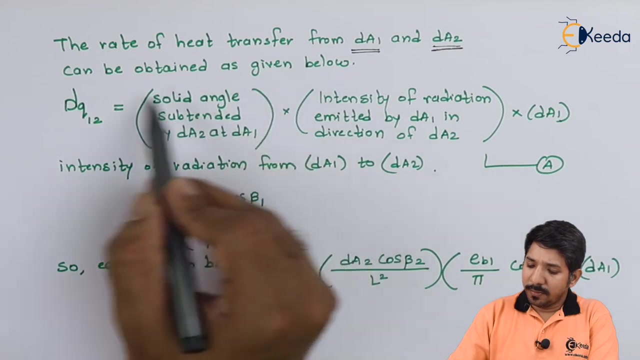 what is the emissivity, or the total emissivity, Then what is solid angle? Now, these three things should be known. to go further with this analysis, The rate of heat transfer from DA1, that is, the small elemental area, to DA2.. Now this can be given as below expression: Now, this is simply a small elemental heat. 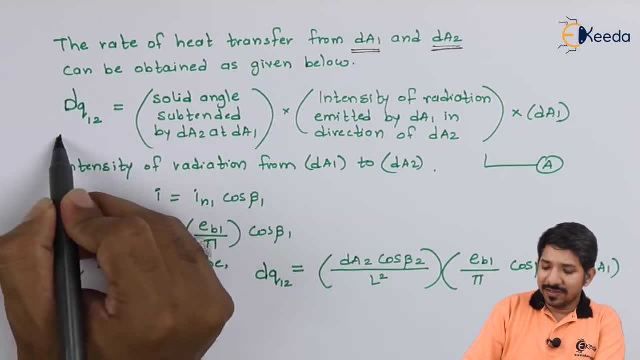 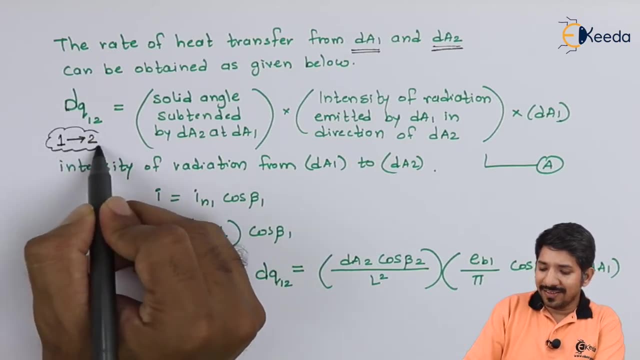 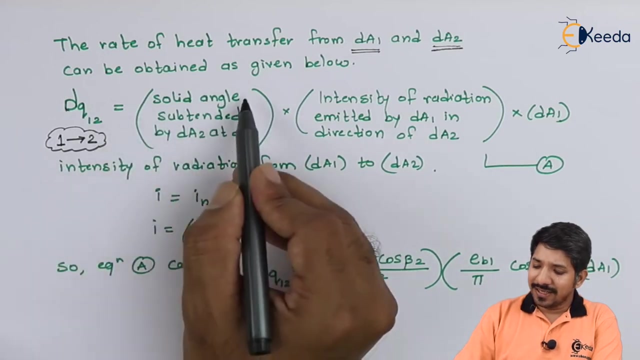 transferred from body 1 to 2.. Try and understand. here we have to consider that heat is transferring from surface 1 to surface 2.. Now for this assumption. we are to trying to find out the expression. Now, with this, the expression itself can be given, as it is nothing but the solid angle. 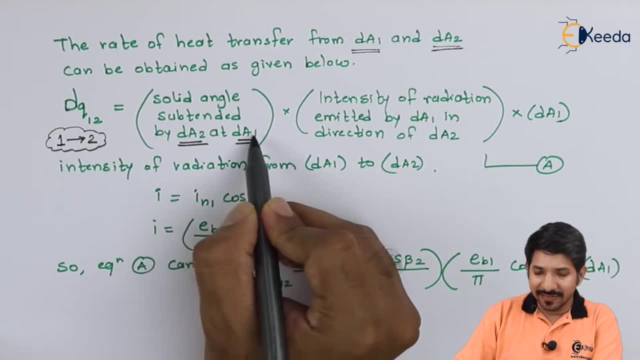 substituted by DA2 at this point: 1.. Now here, according to the results of B2 Simmons, is definitelyiao gain Now, for which we can denote that the touched locations, This infrastructure also has the angle, since relatives D. after that we can dA1, since we are interested in finding 1 to 2, and then the intensity of radiation emitted. 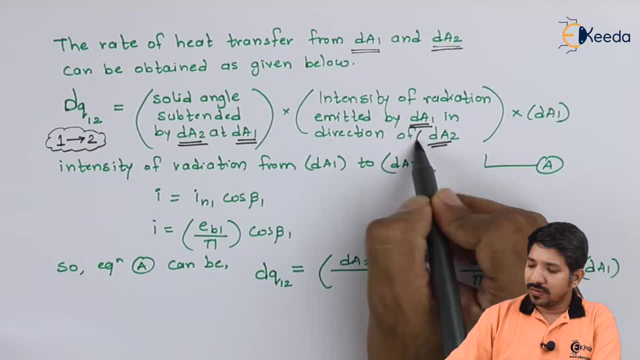 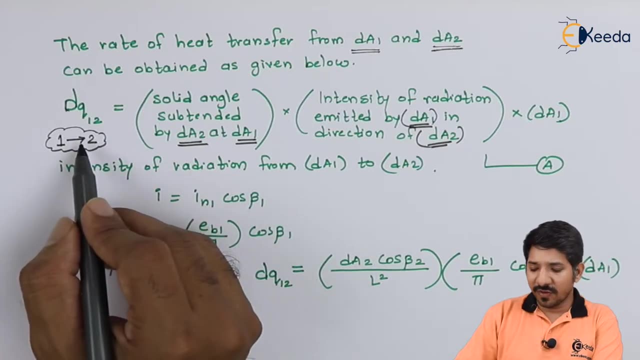 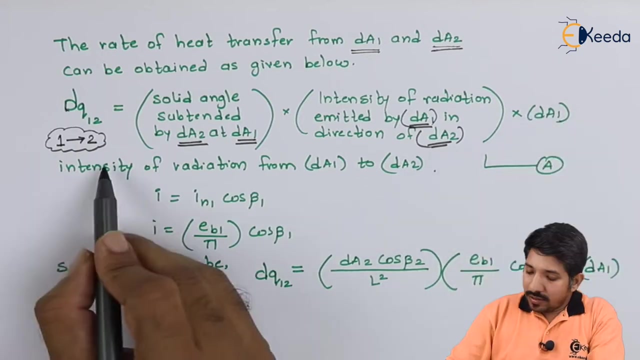 by dA1 in the direction of dA2.. So now, this is what we need to take care of while understanding the heat that is transferring from surface 1 to surface 2: multiple. obviously, the area is the surface 1, that is dA1.. 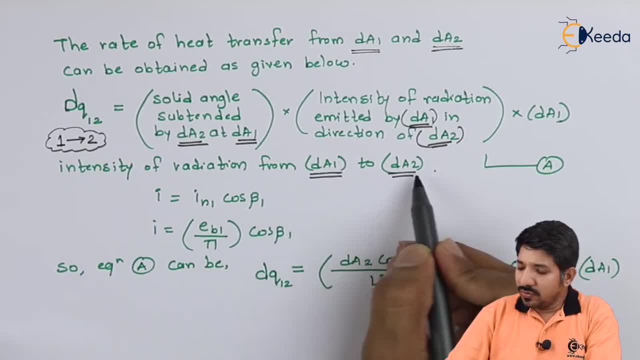 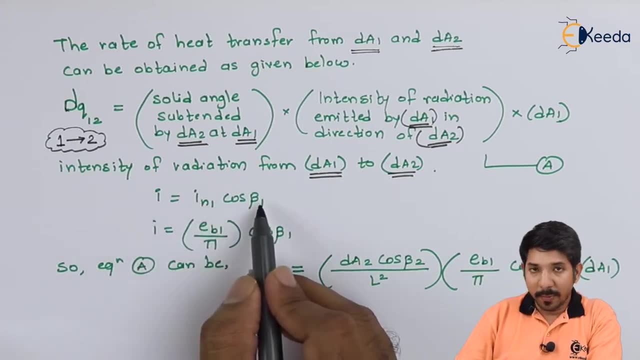 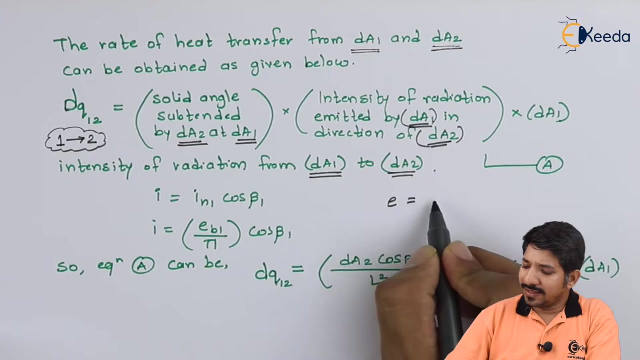 Now the intensity of radiation from dA1 to dA2. this itself is given by the Lambert's cosine rule, that is, I can be written as I of n into cos of V1, then I of n itself can be given. we have seen before that E is nothing but pi into I of n. 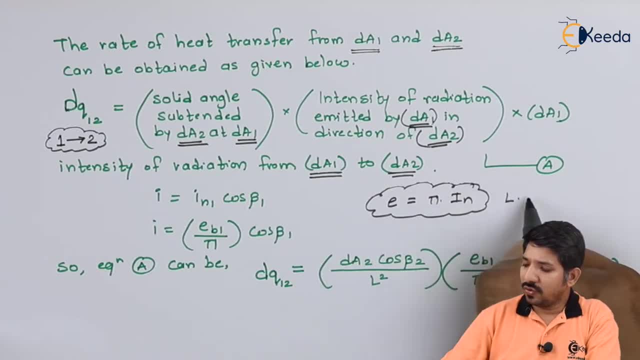 Now, this is what we have seen in case of Lambert's cosine rule. So, since we have considered the black box, I can write this as E, b1 upon pi for the value of I of n, and then I can simply express the cos of beta as it is. 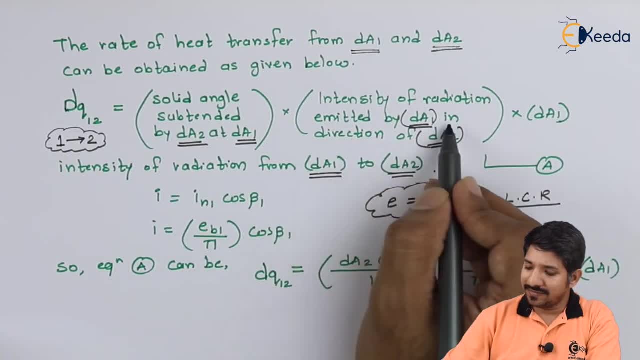 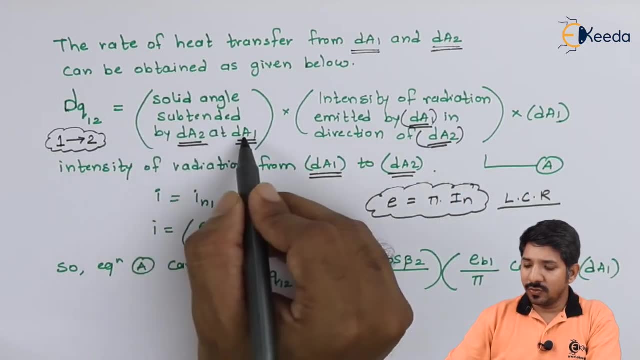 Now, this is the expression for the intensity of radiation emitted by dA1 in the direction dA2. similarly for the solid angle. we know that solid angle subtended by dA2 at dA1 can be written as dA2 into cos. beta 2 upon the distance between the two area is nothing but. 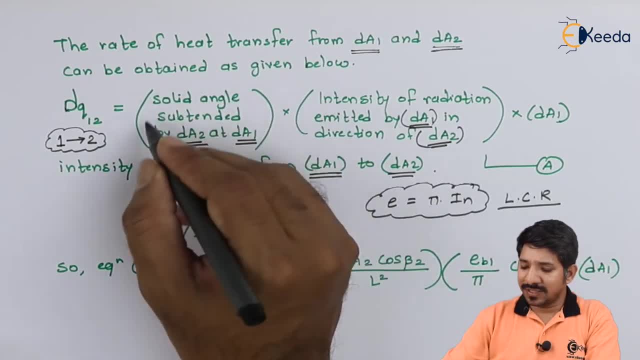 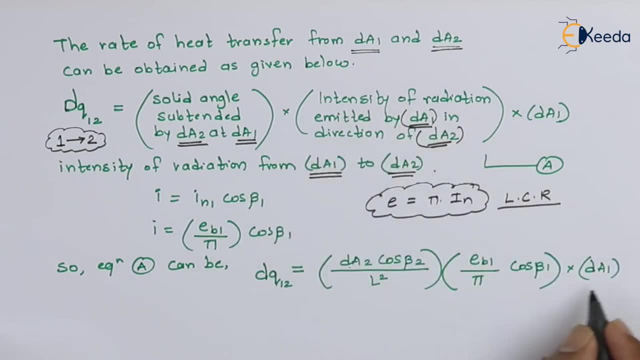 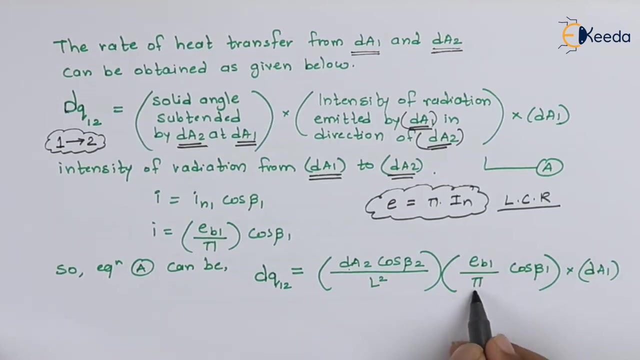 L square. So basically we try to write down the expression For individual statements, that is, for the solid angle and then for the intensity, So we can get the expression something like this: Now let us try to simplify the same expression. See here: in the denominator we have pi L square, and in the numerator this dA1 and dA2 can. 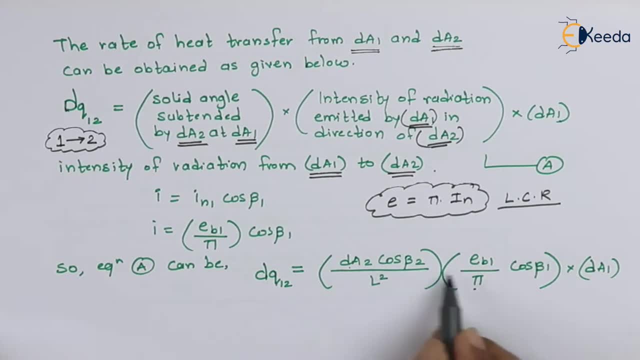 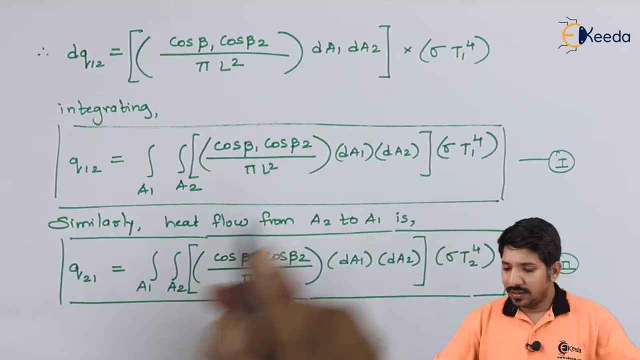 be clubbed together. We have got this E b1 outside and inside we have got cos of beta 1 and cos of beta 2.. Now this was given for a small elemental area, So we can Integrate it. Now, since we have got two areas, that is, dA1 and dA2, it will be a double integration. 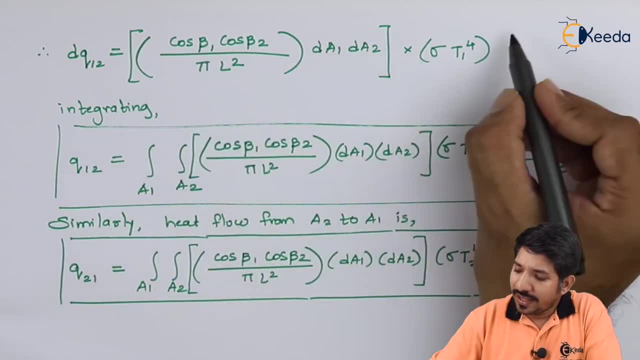 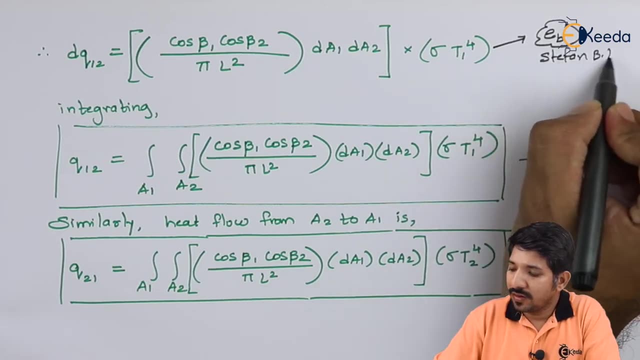 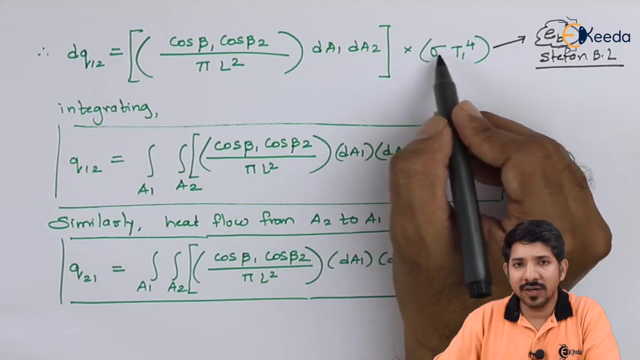 Now that is what we have done here. whatever I have said Now, instead of E of b we have used the Stefan Boltzmann law to express E of b as sigma into t1, raise to 4.. Now, since we have a black body, there is no emissivity or the area is already there in. 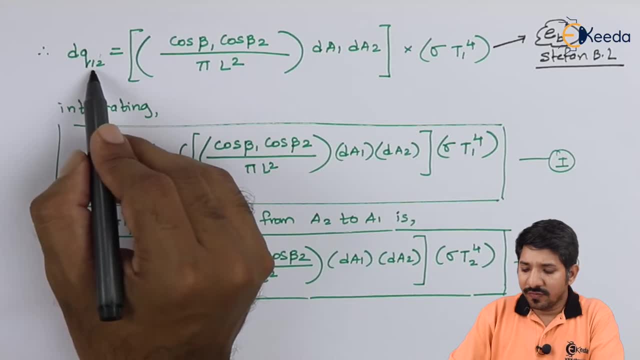 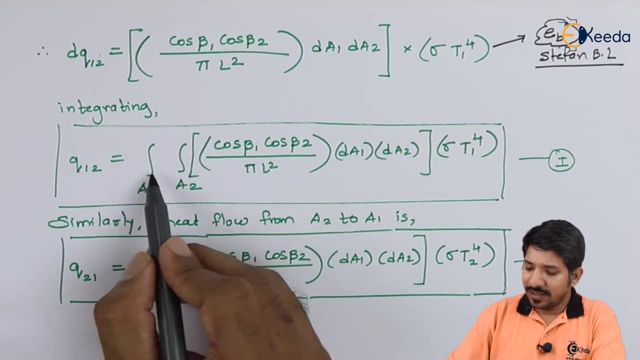 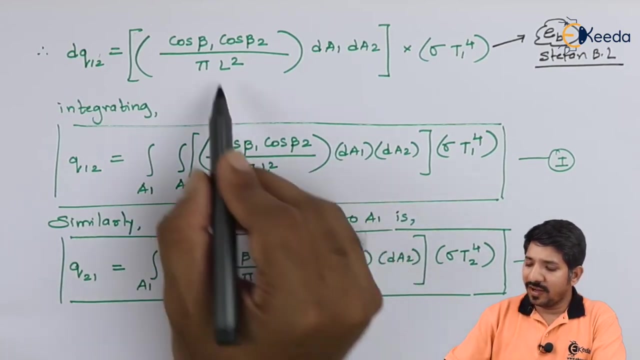 the picture. So that is the value of d of q for 12.. Now by integration we can write the same statement as something like this: Now here it can be written as q1 of 2, as area A1, into area A2 in the bracket we have got. 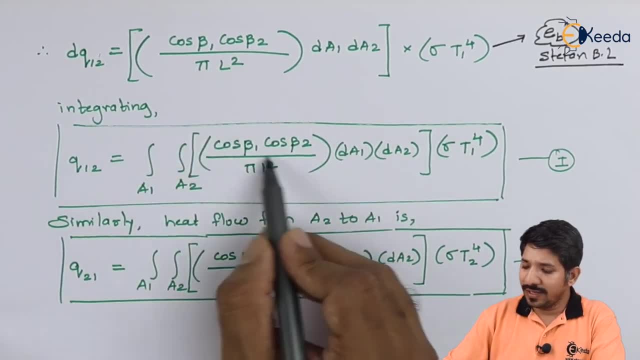 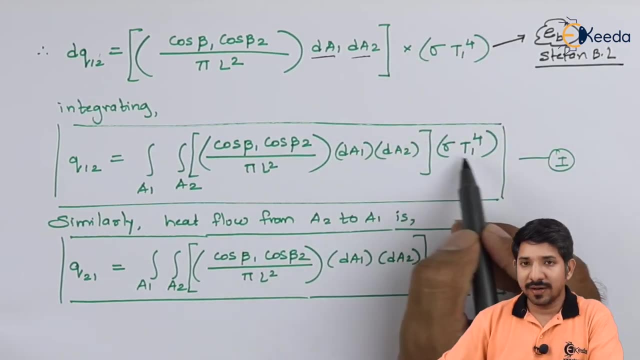 cos of beta 1, cos of beta 2 upon pi L, square in the denominator into the small, two elemental areas. And now what we have done? we have taken this outside. that is, sigma t1, raise to 4. we have taken outside. Now let us write down this as expression number 1.. 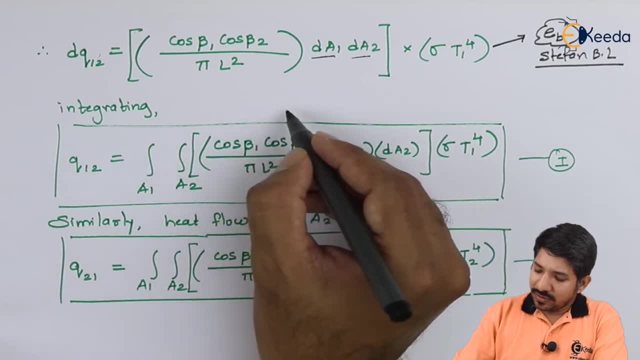 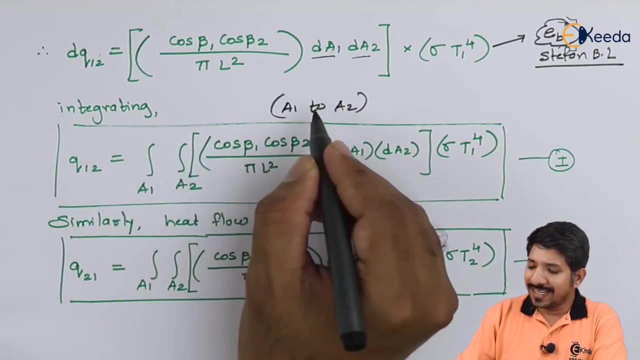 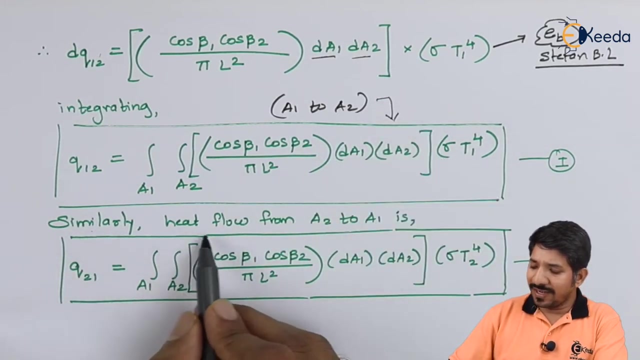 Now, previously we tried to find out that what is the area A1 to area A2.. So the amount of heat that is transferring from A1 to A2 is what we have got over here. Now, similarly, what we can do, we can find out the heat flow from area A2 to area A1.. 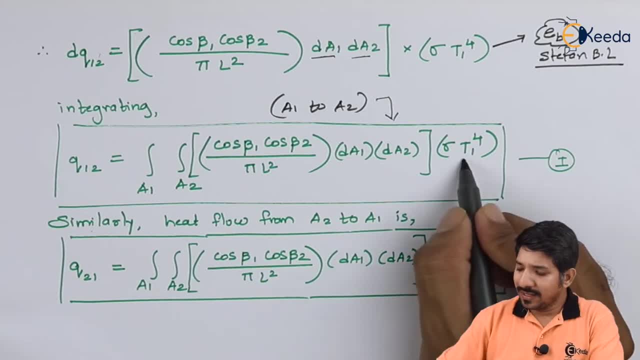 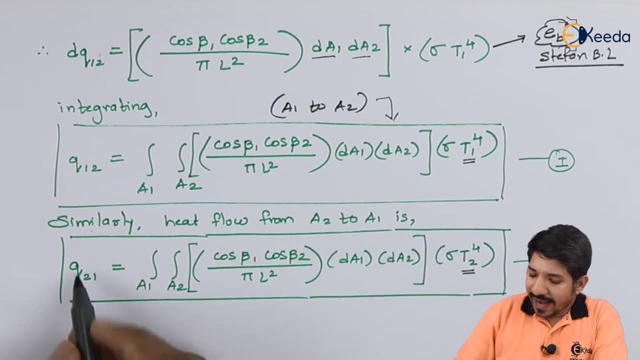 Now, in that case again, everything else will remain same, only this temperature. instead of t1 raise to 4, we will have to write down t2 raise to 4.. That is the only difference over we have. And one more thing is that instead of q1 to 2, we can write down this as q2 to 1.. 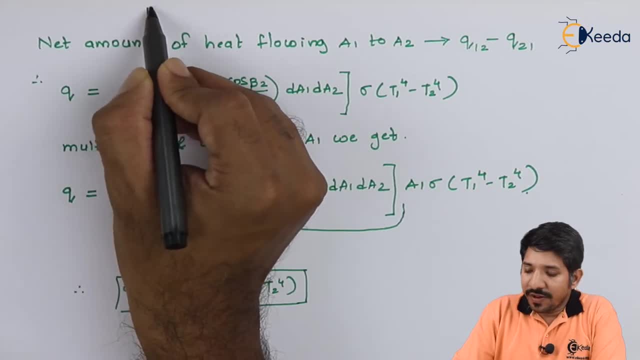 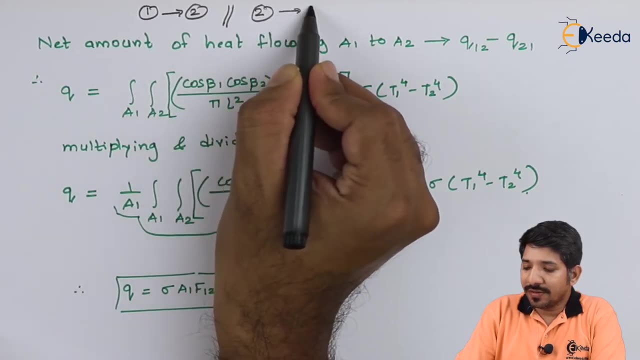 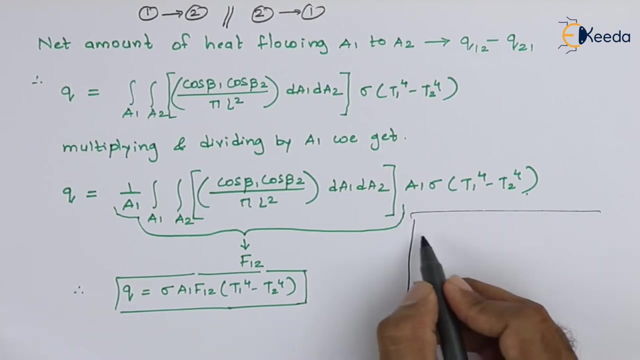 So what we have found out? what is the amount of heat that is transferring from body 1 to body 2.. Similarly, what is the amount of heat that is transferring from body 2 to body 1.. So we need to understand that there are two ways by which the heat will be transmitted. 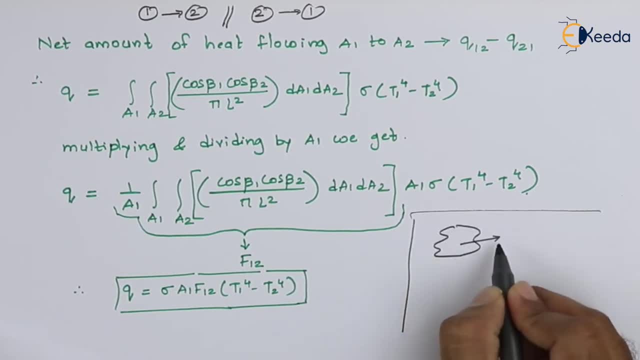 A body. if a body itself is emitting heat Or radiation, those can be of its own, that is its own emission, or it can be reflection. So what is reflection? Reflections are nothing, but some other energy is coming onto this body and it is reflecting. 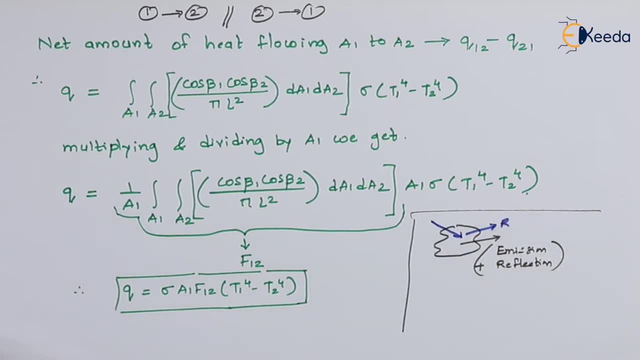 So one is due to reflection and the other one is due to emission. Now for this. if I need to find out the net change, The net change, The net change can be found out by taking the difference of the two. Now, that is what they have done. 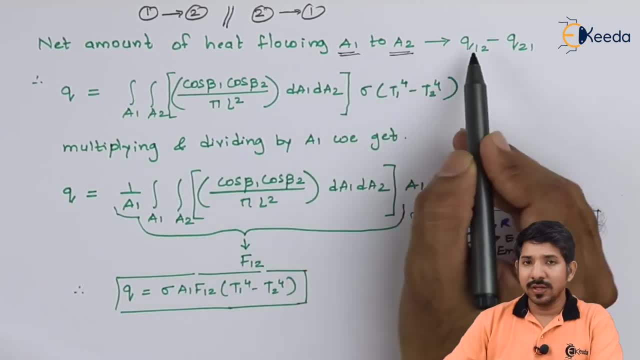 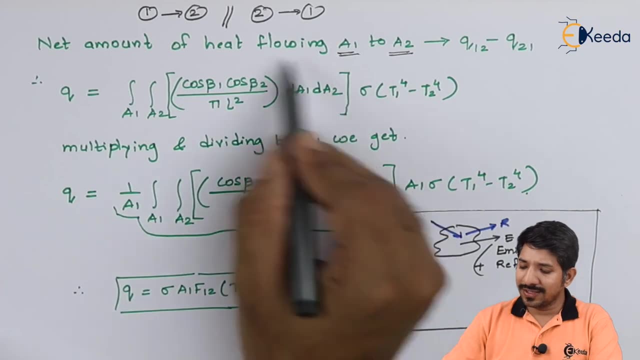 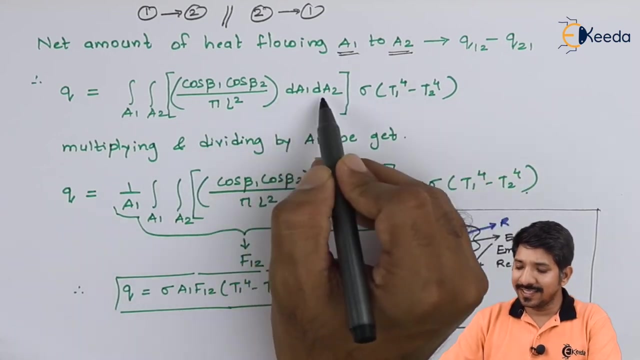 The net amount of heat flowing from a1 to a2 can be found out by this: That is q1 to 2 minus q2 to 1.. So with this, again, all the other things are constant. What they have done, They have taken out this t1 and t2 outside the da1 and da2.. 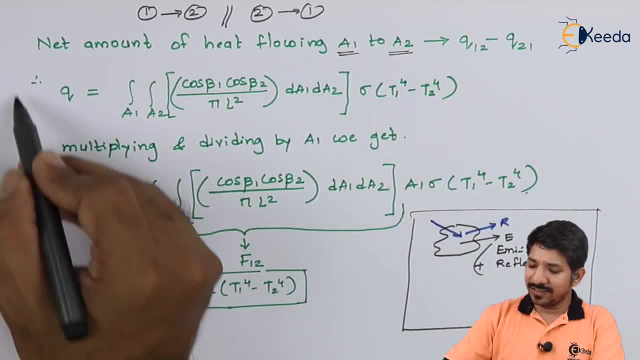 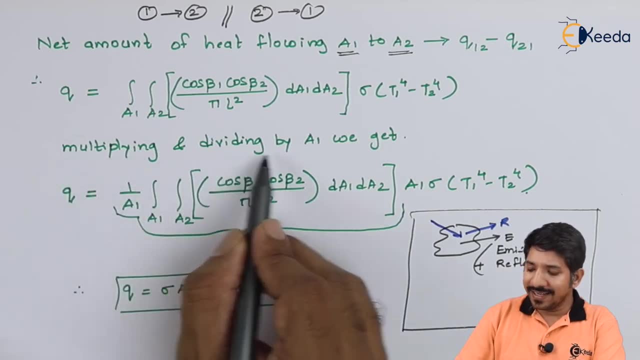 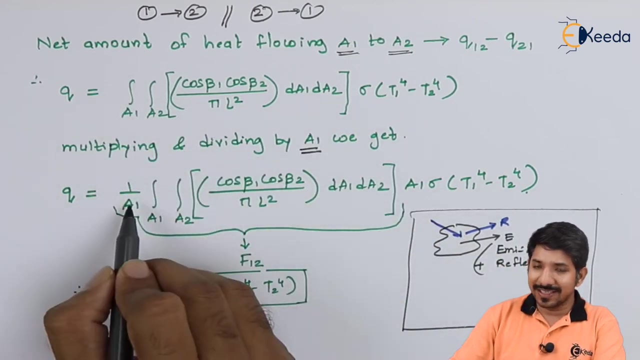 If they can do this, then I am having the equation something like this here Now. in this, What modification we are doing is we are simply multiplying and dividing by area a1.. So what do we get? We have here 1 upon a1, that is, outside the integral bracket and inside, obviously, we again. 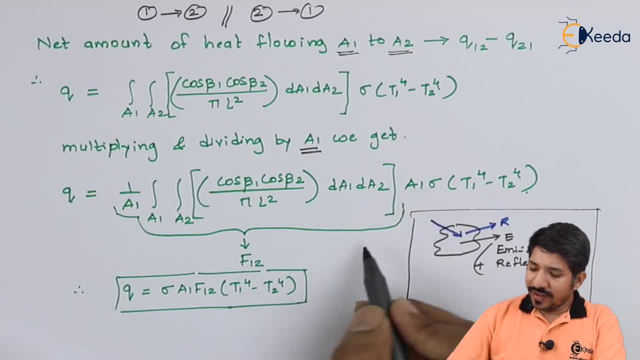 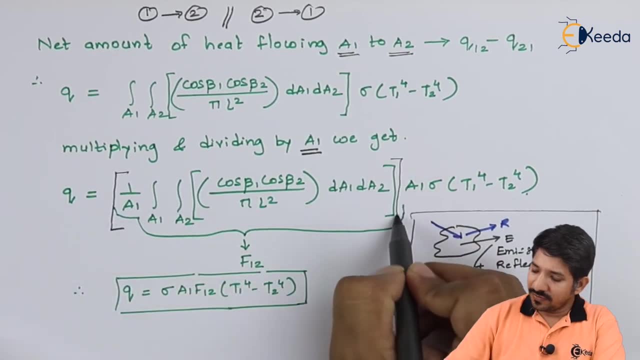 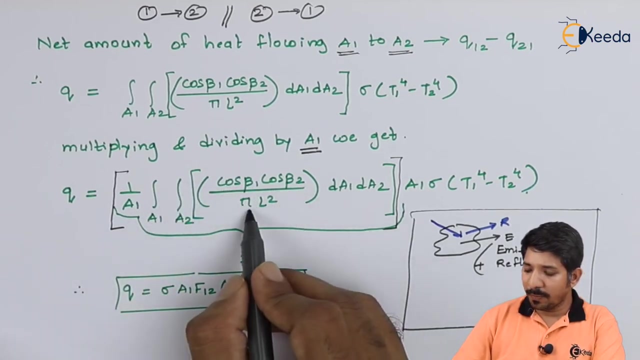 put one more a1 over here. Now, what do we have At the end of this expression? this entire term, see here, starting from 1 upon a1. integral a1, integral a2.. Close Cos of beta 1. cos of beta 2 upon pi. L square into da1 and da2.. 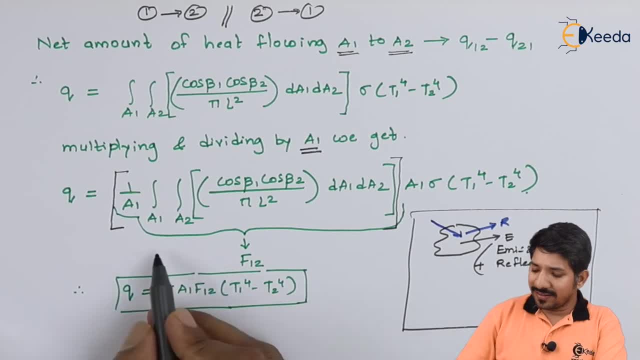 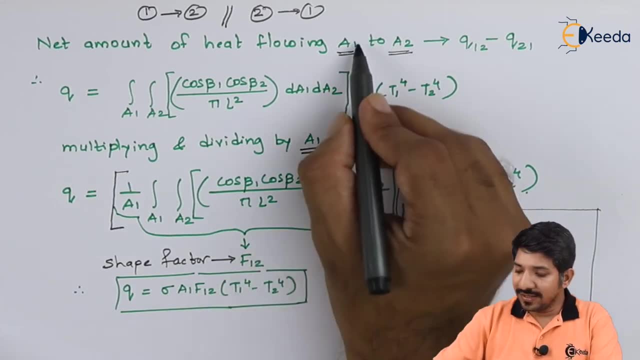 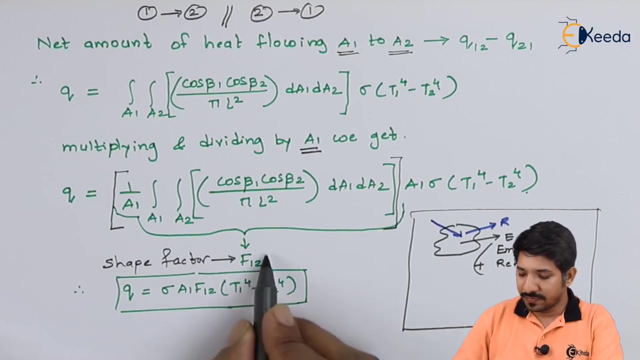 Now this double integral itself is called as a shape factor. Now, since we are talking about from 1 to 2, this is written as f1 to 2, that is, shape factor of 1 for surface 2.. Now this entire expression is given as shape factor 1 to 2, and it can be observed. 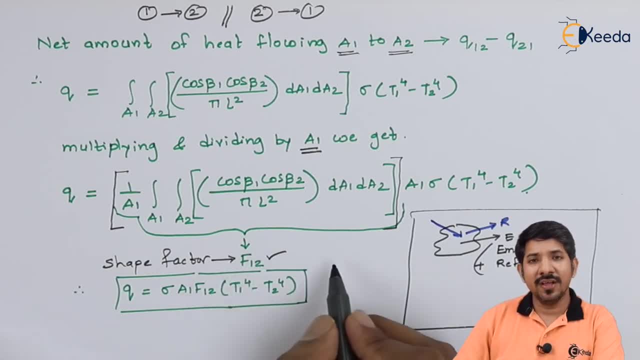 Or it can be found out by various expressions or some charts. There are typical charts are available for standard shapes or some sort of a tables are available, So using those we can find the value of the shape factor. or we can simplify this Q itself as writing. Q is equal to the Stefan-Buhlmann constant sigma into a1, into f1 to 2 t1 raise. 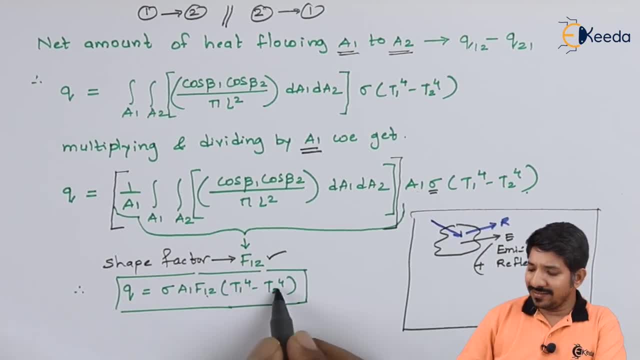 to 5.. So this is the shape factor. So this is the shape factor. So we get here: f1 to 4 minus t2, raise to 4.. Now this is the final expression that we have for the heat transferred from one body to. 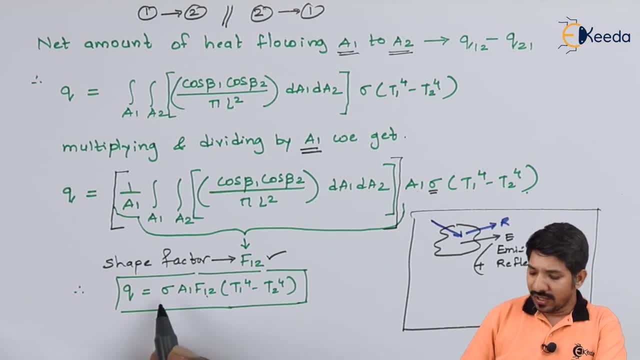 another body by considering the given body as a black body. Now, if suppose instead of a black body we have a gray body, then obviously one more term will come into picture, that is the emissivity. So emissivity into sigma a1, f1 to 2, t1 raise to 4, into t2, raise to 4.. 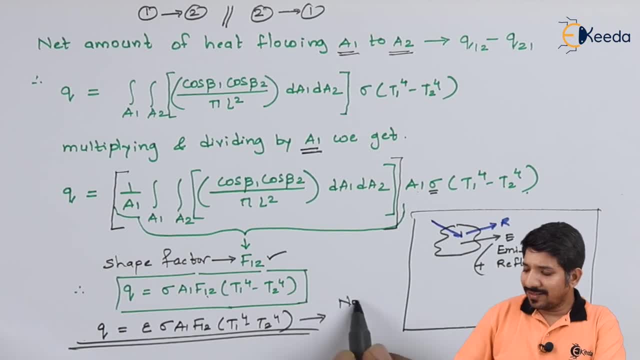 Now this is given for a, So this is the emissivity. So this is the emissivity, So this is the emissivity. you can say that non-black bodies or a gray body, so only a emissivity term will come into picture for any other given body. so in this topic, basically, we successfully find out the.